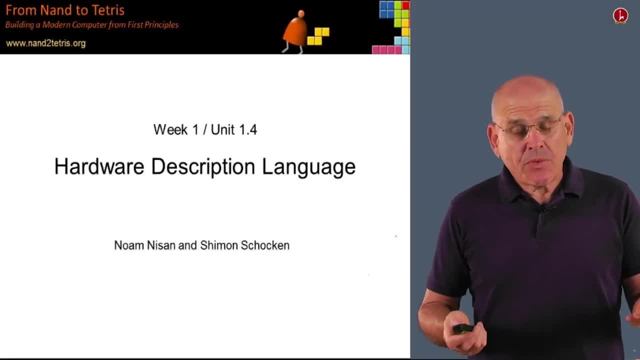 In previous units we talked about how Boolean functions can be realized using logic gates, And in this unit we're going to talk about how we can actually build and implement the logic gates using a formalism called Hardware Description Language, or HDL. 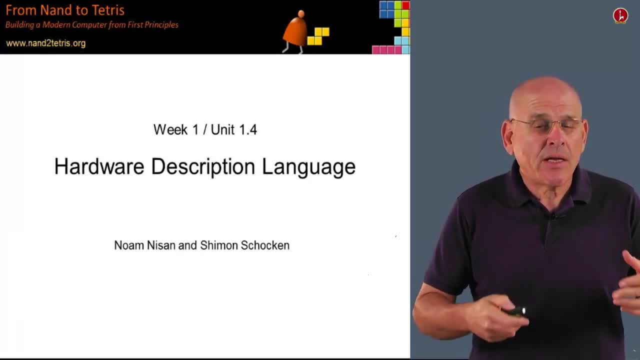 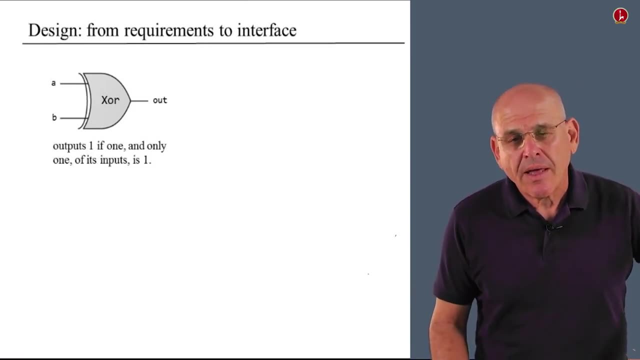 Once you build a logic gate in HDL, you can actually simulate it, test it and finally build it in hardware, as we now turn to describe. All right, so let's begin this journey from obstruction to implementation. The first thing that you have to do as a gate architect is demand. 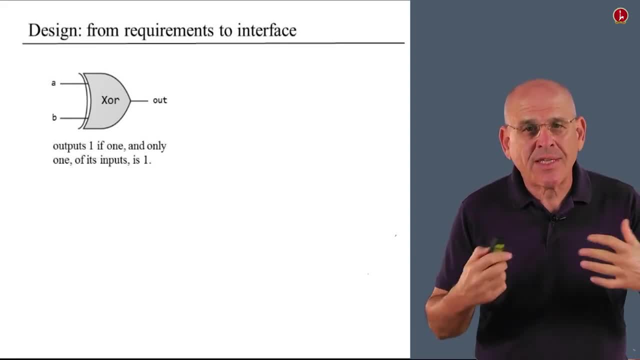 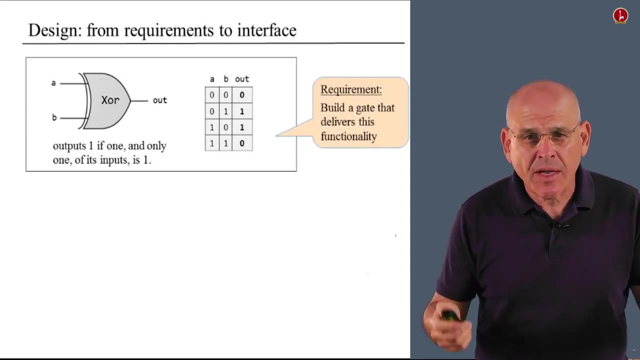 a full and complete description of the desired gate's behavior, And in this case, what we need is some sort of a truth table. In the case of XOR, it's a very simple truth table, And the truth table, along with the gate diagram, gives you everything that you. 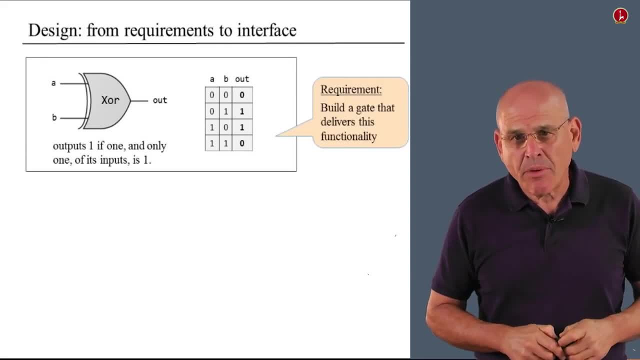 need in order to understand what this chip is supposed to do, And what we see here is also sometimes called the chip's interface, And indeed, using this information, you can start writing an HDL file that will look something like this example here: 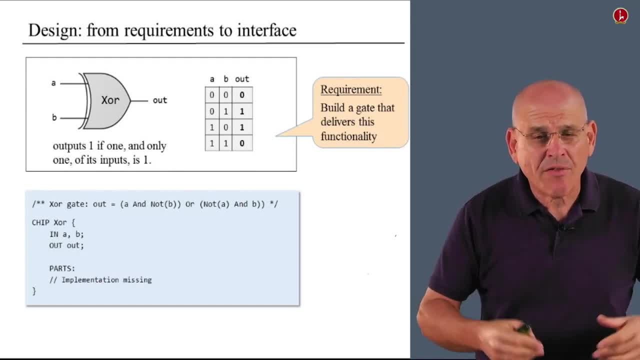 So we start the HDL program or the HDL file, some documentation, free form- You know you can write whatever you want there- which describes what the gate is supposed to do, And then we specify the name of the chip, the names of the inputs of the chips, 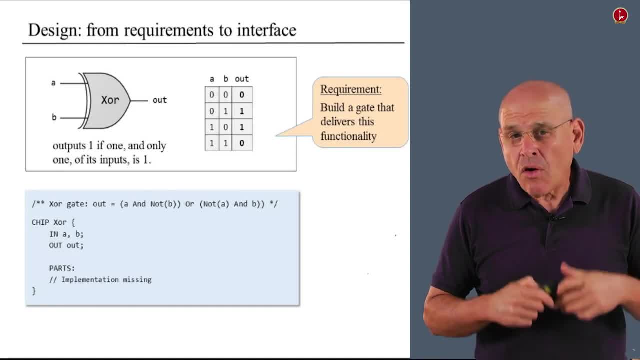 and the names of the chip's output And all this information- by the way, the name of the chip and the names of its inputs and outputs- is typically given to you. You know it's not something that you decide, it's something which is part of. 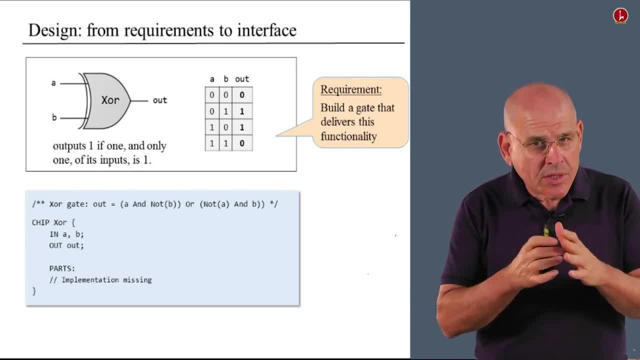 the chip's output Contract, if you will. So you simply write it up using the syntax And then you write the magic word parts which describes that. here begins the segment of your program in which you're going to describe how this chip is actually designed. 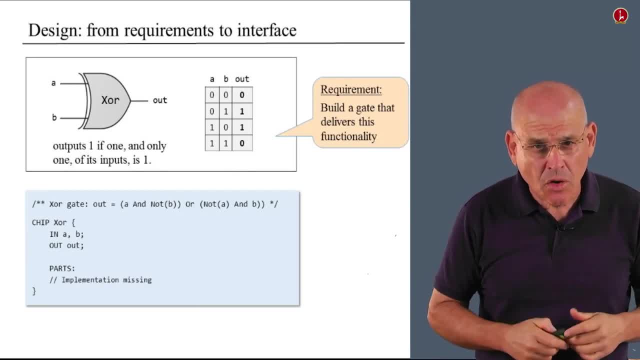 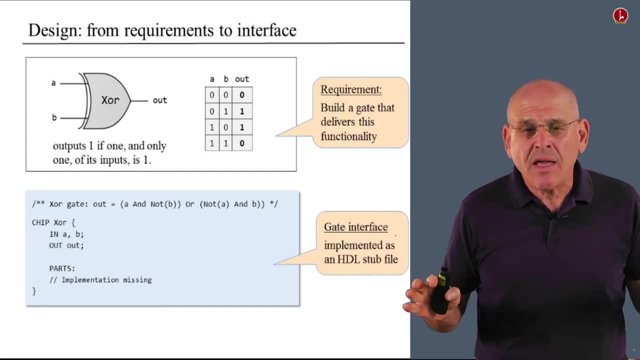 Now, when you use such a chip, such a XOR chip, what we've seen so far is called the gate interface, And notice that this is everything that I need in order to use XOR gate. However, if I have to build this gate, well, that's a different story. 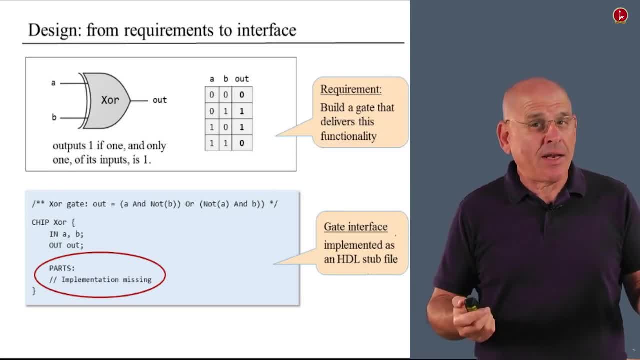 Now I have to open up the black box and actually design it. So when we use chips, we always wear two different hats. There's the hat of the programmer who uses the chip at the chip part, And for this all we need to know is the chip interface. 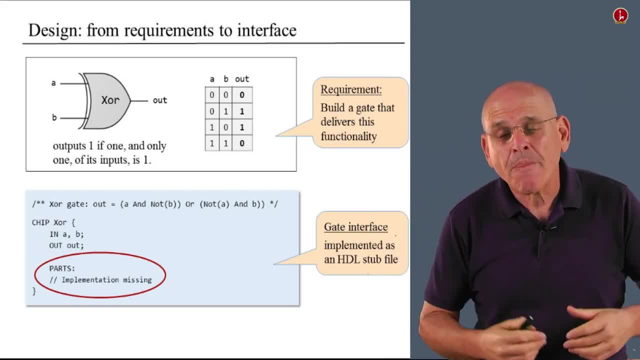 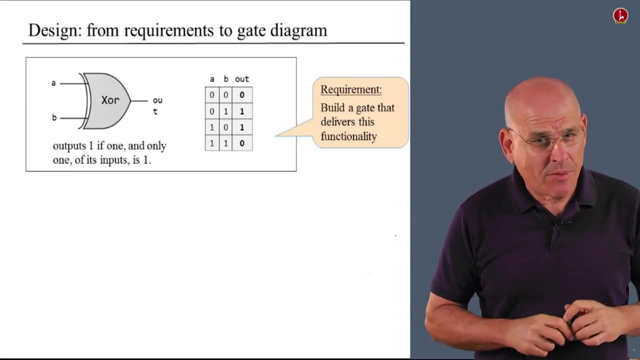 And there is the other hat of the chip's builder, which is what we're going to do now. So, moving along, let's discuss how we actually build this chip from scratch. All right, so actually we are not going to build it from scratch. 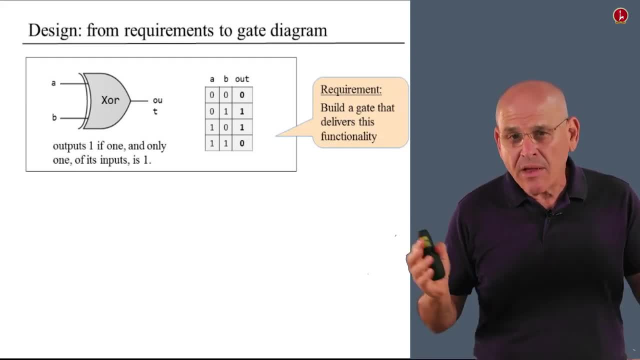 We can, if we, if we need to, we can build it from NAND gates only. However, let us assume that we we've already built an AND gate, an OR gate and a NOT gate. Well, if we built these gates or if someone gave us these gates, 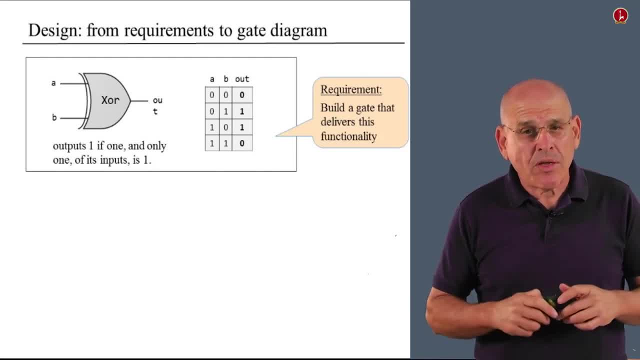 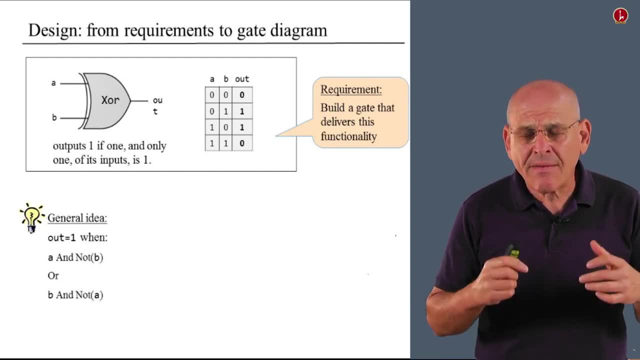 that we can freely use. here is what we can do. We can inspect the truth table and figure out from the truth table that the XOR functionality can be described as follows. I mean, look at the XOR, look at the truth table. 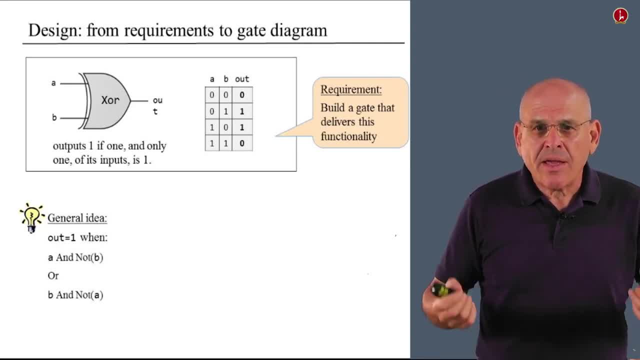 The gate outputs one in two cases only: If if A, if A and not B, or if B and not A, That is, if A is true and B is false, or if B is true and and A is false. This sort of comes out, jumps out from the truth table. 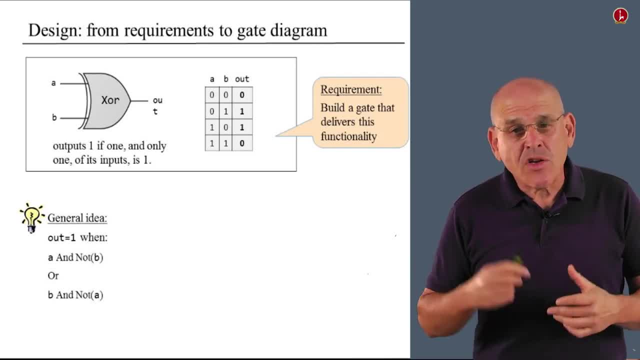 You can either see it on your own or, as Noam described in one of the previous units, you can synthesize this, this insight or this Boolean function, from the table itself. So once you come up with this insight, the next thing that you do is you think about it for a little while. 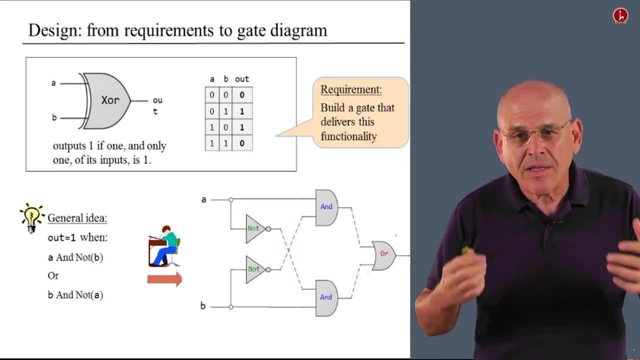 And you come up with a gate logic diagram that describes how we can build this Boolean function using basic logic gates that we already have to our disposal Now, developing such diagrams is a matter of experience, And the only way to to gain this. 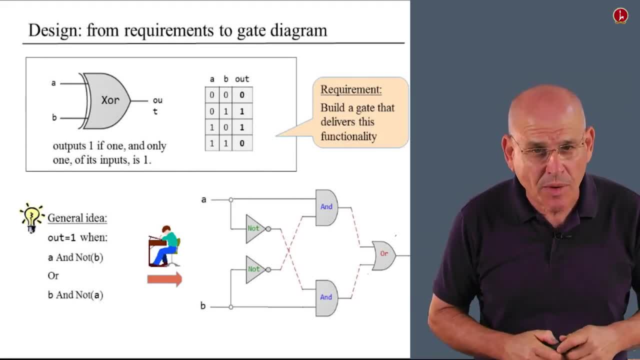 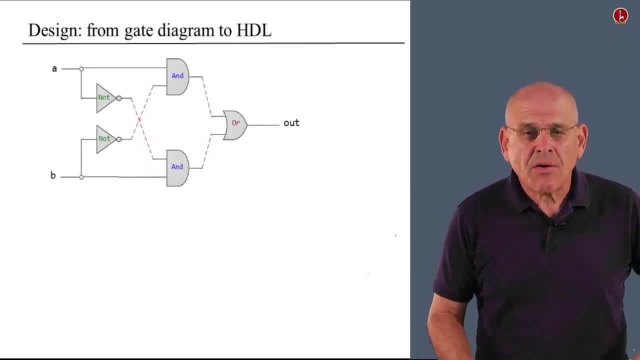 this expertise is to see many, as many examples like like this one. So let's take this example and and explain it in in detail. So the first thing that we can do is draw the boundary of the chip diagram, Now the, or the gate diagram. 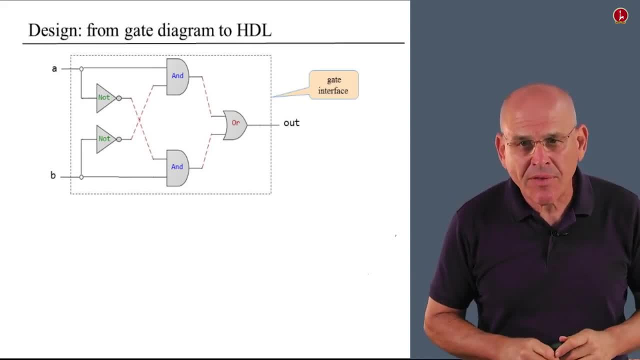 So we use this dashed outline for this purpose, And what remains outside the boundary is the use of the gate User's view of this gate, In other words, the the gate interface. All the users knows is that he or she has a gate that has two inputs, A and B. 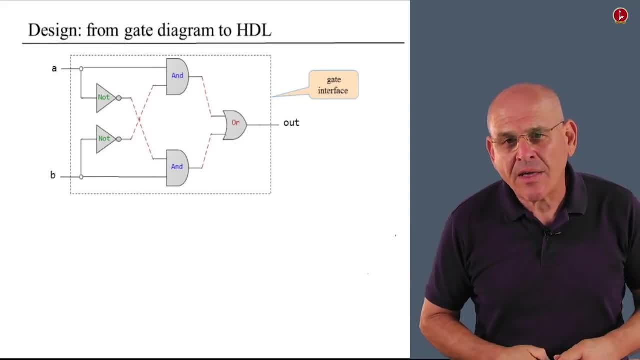 And output called out, And all together they somehow this chip, as if by magic, delivers the XOR functionality. So we draw this diagram and and this interface, And now we can delve more into the, into the inner architecture. So notice how the A signal is being. 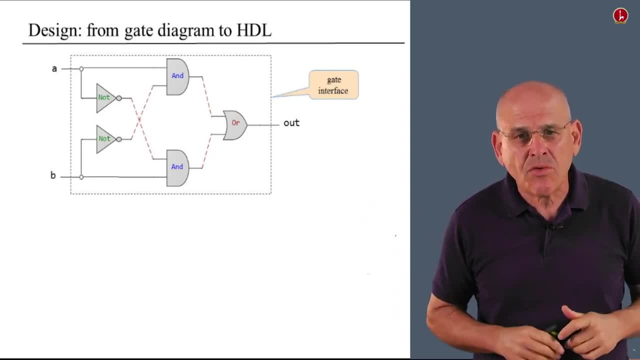 copied and sent simultaneously into two different destinations. One of them is the end gate and the other one is a, not gate. This is perfectly okay in chip diagrams And we see that the B signal undergoes the same, the same treatment, And in general when you write HDL code. 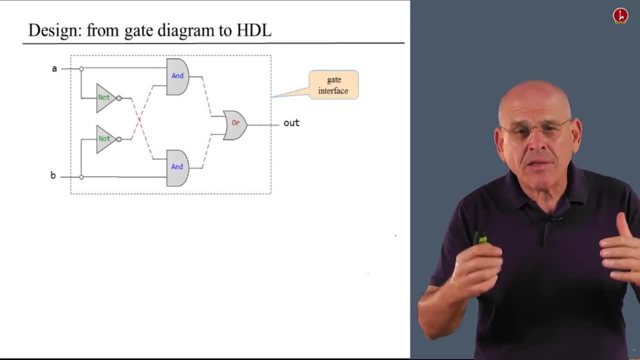 you are allowed to take any signal and distribute as many copies as you want of this signal into as many destinations as you want. This, this wiring or these dispatching is done simultaneously. So, to use a formal language, HDL has unlimited fan out. 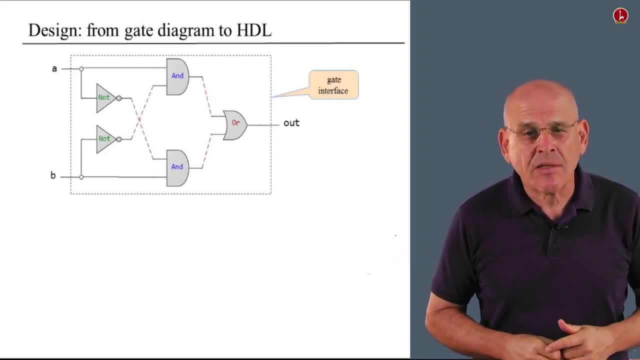 You can. you can fan out any given signal to as many destinations as you want And we do it. We always do it when we write HDL code: All right, moving along. notice that we're using some off the shelf gates. 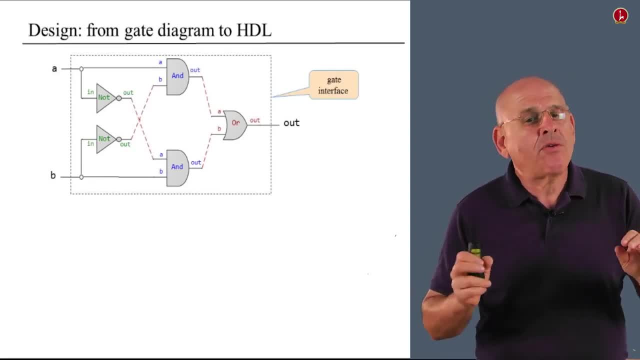 And not and or. Now, whenever you use an off the off the shelf gate, you are bound to use the names of the gates: input and output as advertised, so to speak. In other words, when you take the gate gate off the shelf, the gate comes. 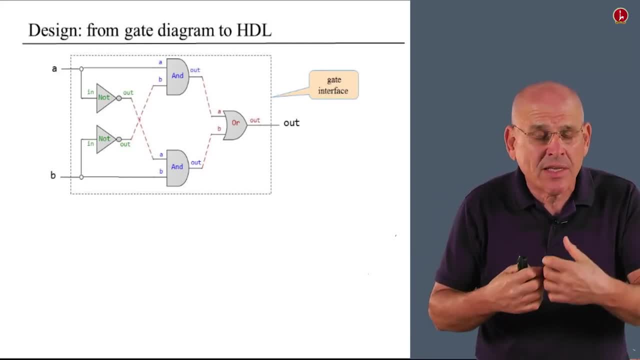 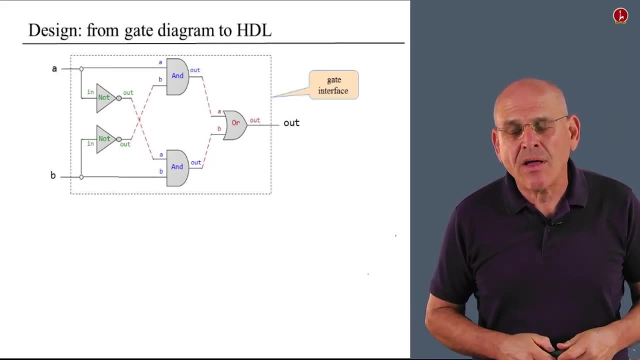 along with what can be called the gate signature or the gate's API. So we have no degrees of freedom here. We have to use the official names of the, the inputs and outputs of of every one of our chip parts. Now the next thing that we do is let's focus on the red connections that we see here. 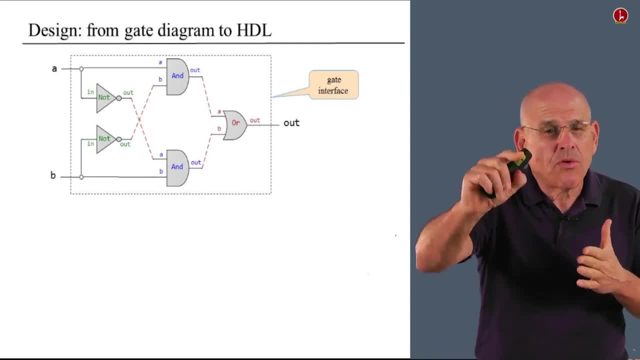 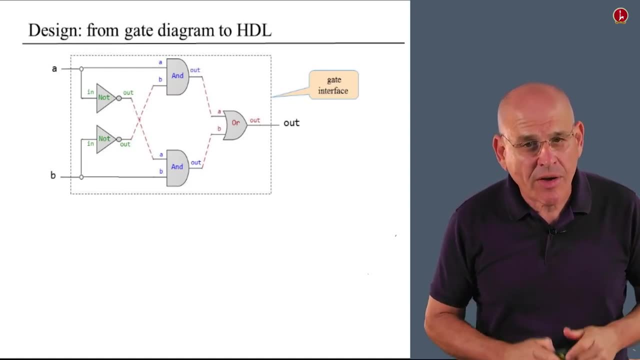 These are the connections that we draw in order to connect the different chip parts together. Now, the rule is that every one of these connections has to be named, And it's our responsibility to come up with sensible names, So that's what we do. 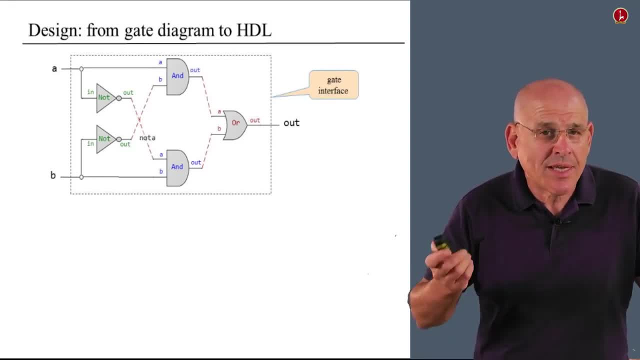 We can call this particular connection not A, which is a sensible name, I think, A self-descriptive name. We'll do the same thing with not B. We can call this one A and not B. We can call this one, not B, not A and B. 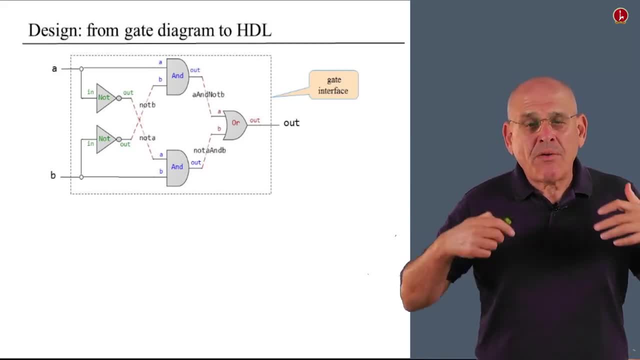 And and that's it, We. we, we have named all the internal connections in our architecture And we can actually now move on to describe this diagram in HDL. So now we can actually move on and implement this diagram using HDL. 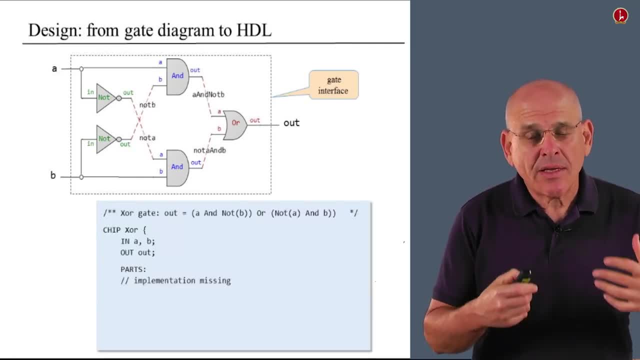 So we return to the HDL stub file that we had before, And I used the table- the term stub file- to describe a partial HDL implementation, so to speak. that actually describes only the chip's interface And typically it comes with the the statement implementation missing or 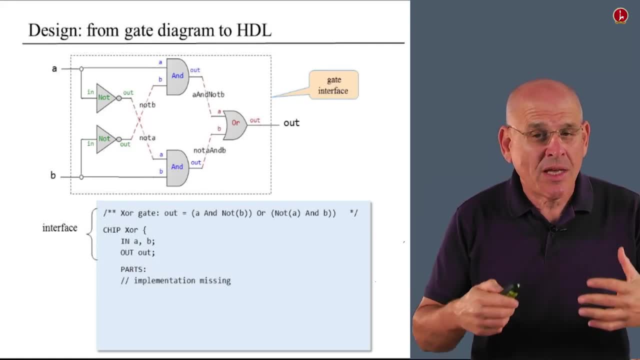 put your code here, and so on and so forth. So this is the contract that we actually have to implement, And now, indeed, we are going to focus on the implementation section of this file And basically what we do is we begin to describe. 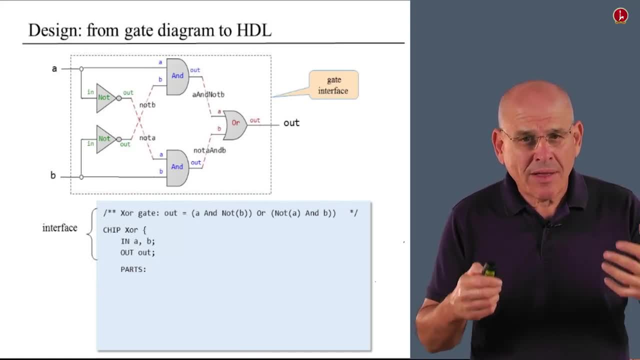 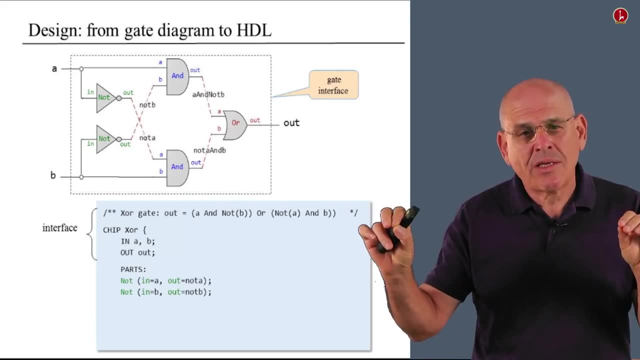 the gate diagram, one chip part at a time, And for each one of the chip parts that we have, we write a single HDL statement that describes the chip along with all its connections. So we have two. we happen to have two not chip parts, so we describe them. 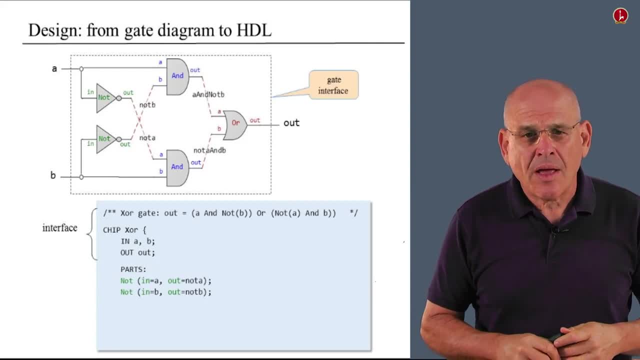 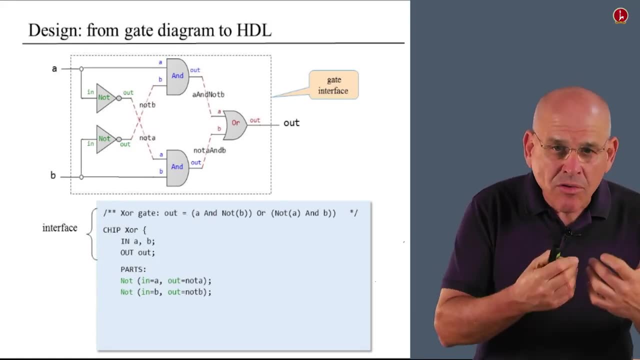 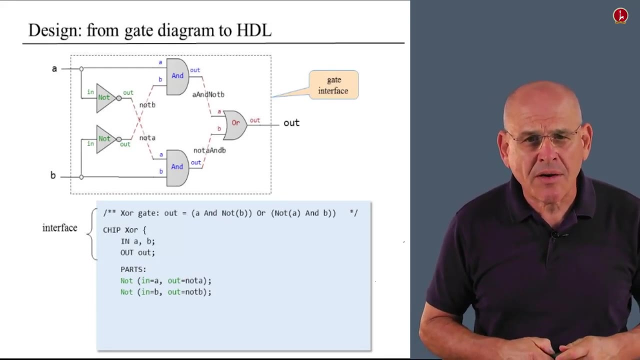 The first, not has. n equals a. This is the input. you know the, the in input of the chip receives the, a signal, And the out output of of the chip goes into, not a. We do something similar with the with the other, not chip. 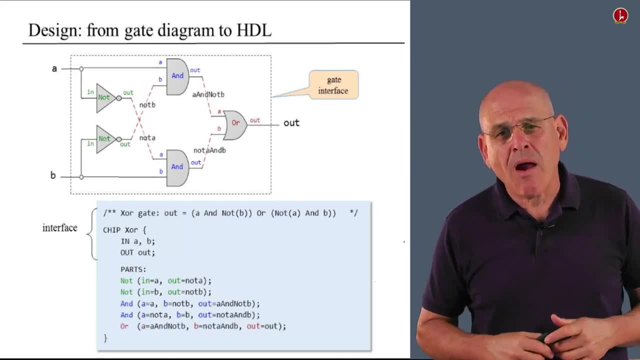 Then we describe the two n chips and finally we describe the the all chip. Notice, by the way, that I use the words gate and chip interchangeably, And that's perfectly okay. A gate for me is simply a simple chip, All right. so this HDL diagram is nothing more. 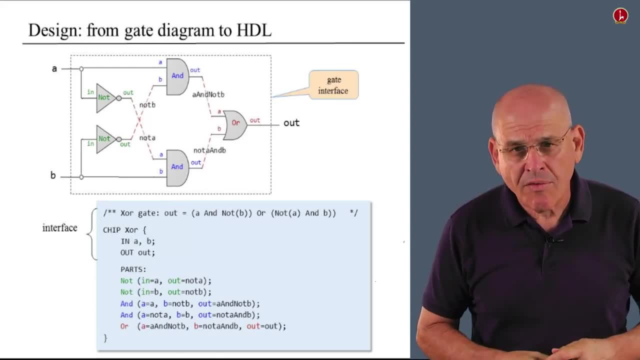 than a textural description of the gate diagram. Did I say HDL diagram I? I meant the HDL file is a textural description of of the gate diagram that we see at the top of the slide. Now I'd like to to notice that once again we have interface. 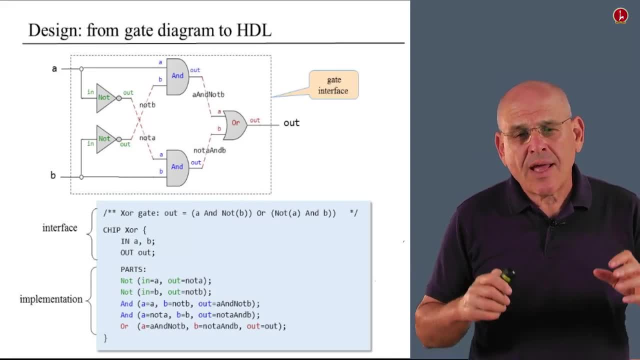 We have implementation And also note that the interface of the chip is unique. You know, there's only one way to describe this chip, And this is typically given to us by whoever you know commissioned us to implement this chip. At the same time, the implementation is not unique. 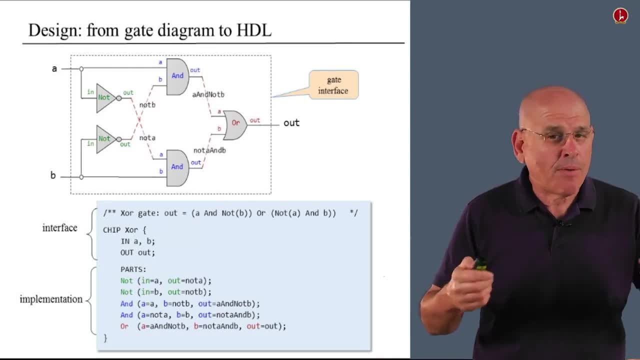 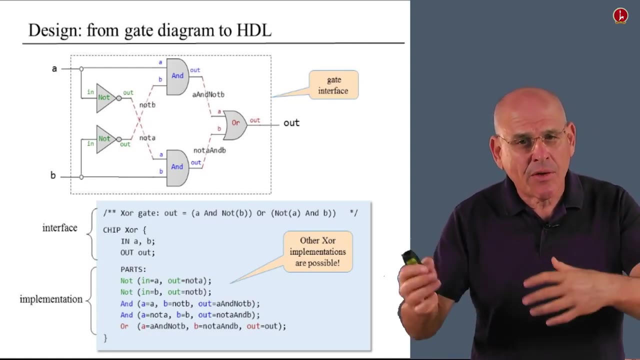 And the same interface can be implemented in typically in many, many different ways. for example, in the case of XOR, we can implement the XOR chip using three logic gates only, So and it doesn't really matter how exactly we do it. 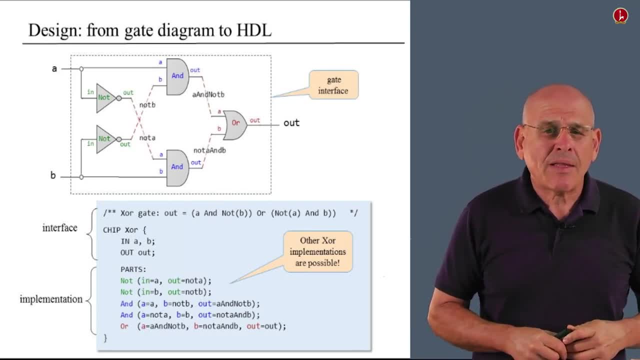 We can. you can think about it on your own if you want, But in general there may be different implementations and some of them will be less expensive. They will contain less chip parts, less connections, consume less energy, and so on and so forth. 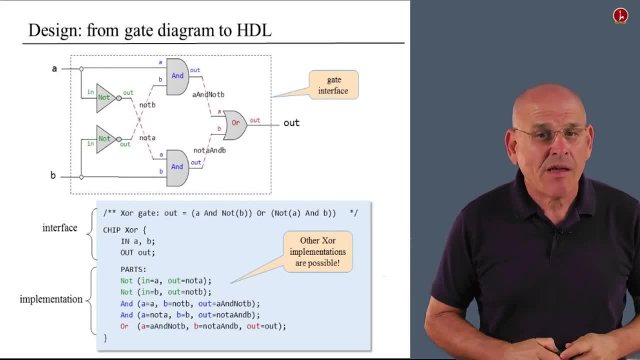 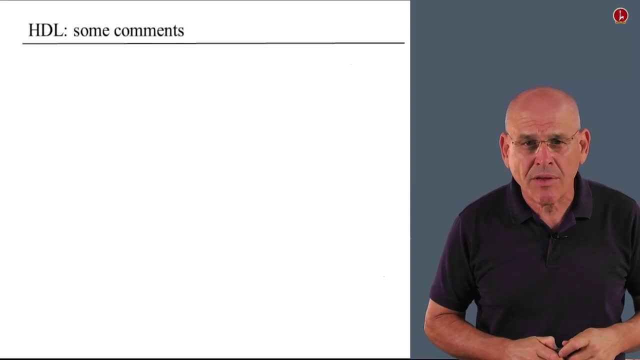 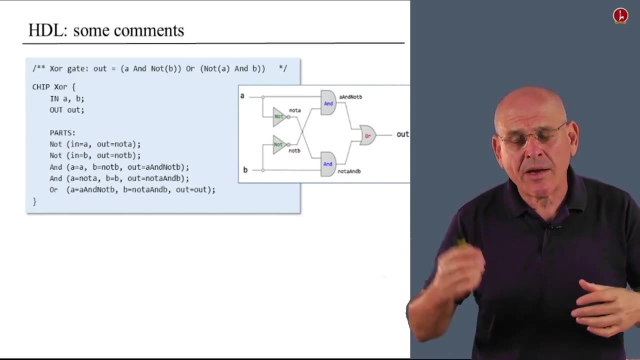 So the interface is unique and the implementation varies. Now I'd like to use this opportunity to make some general observations about about HDL, And, for ease of reference, I have placed in front of you what we saw earlier in this unit: the, the gate diagram on the right hand hand side, and 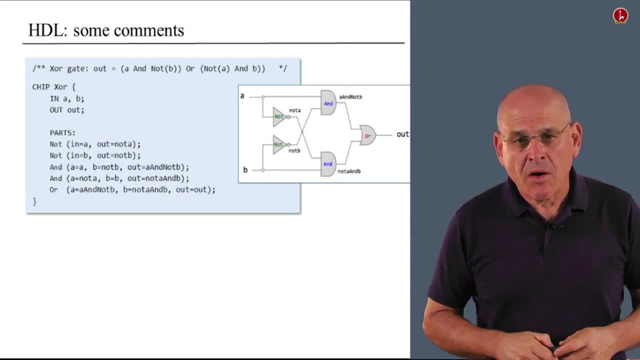 it's HDL description on the left. So what? what can we say about? about HDL? First of all, we see that there are certain issues in HDL which are very similar to what we normally do in other programming languages. 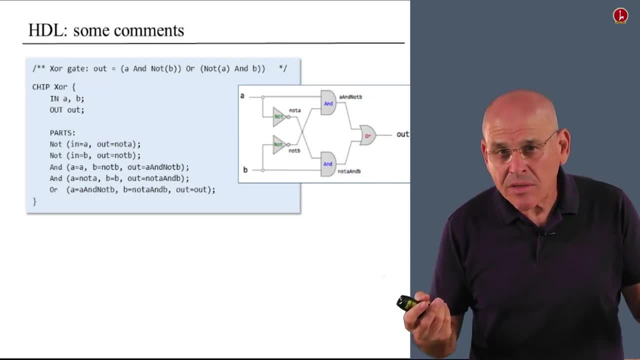 We have to worry about good documentation of our HDL program, just like we do when we write a program in Java or Python. We have to come up with good descriptive names both to the chips that we use and to the Connections that we, that we create within the architecture. 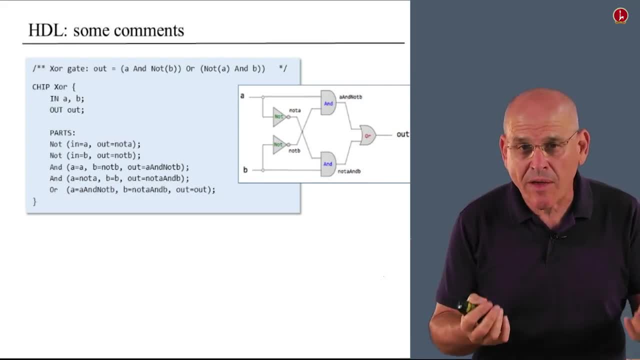 So readability is terribly important. You know, we have to make sure that our HDL code is self-descriptive and readable, And in order to do it, we also use indentation, you know, and and make the code look real nice. 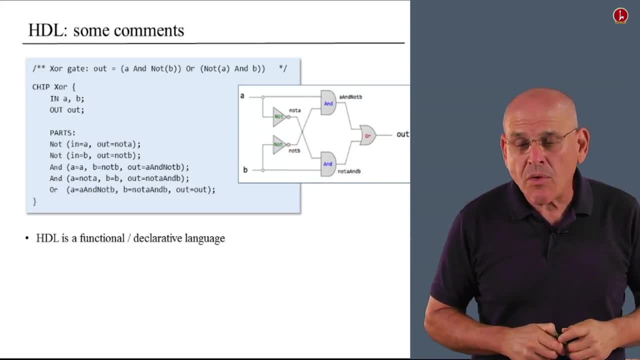 So all these things are expected from you when you write your own HDL programs. In addition, there are certain things which are really unique to HDL. First of all, HDL is a functional or declarative language. There's no procedure going on. 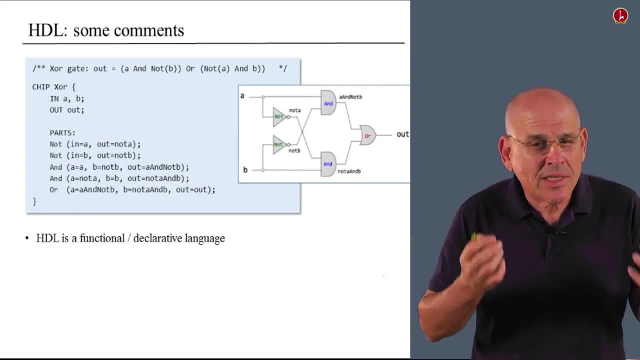 There's no program execution going on. It is nothing more than a static description of the gate diagram. At the same time, you know we assume that at some point this descriptive code will go into some interpreter. You know it will go into, in our case into a hardware simulator that. 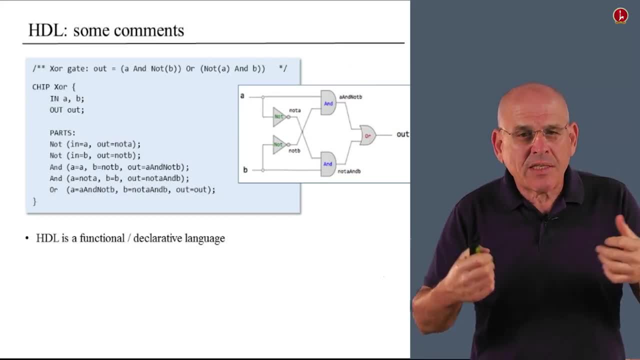 that can actually take this description and start to sort of pipe values From the bottom all the way to the end. So we assume that there is some agent that will turn this implementation into something that is actually working. But this procedural part is not part of the HDL code. 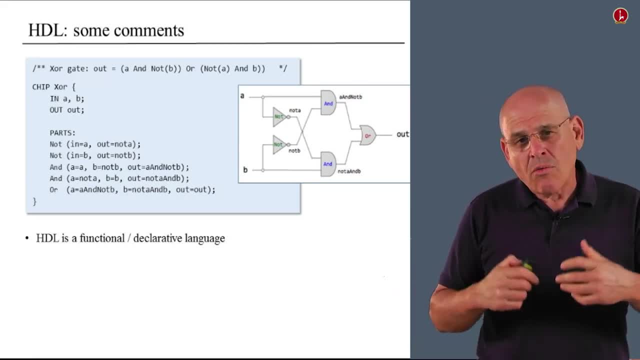 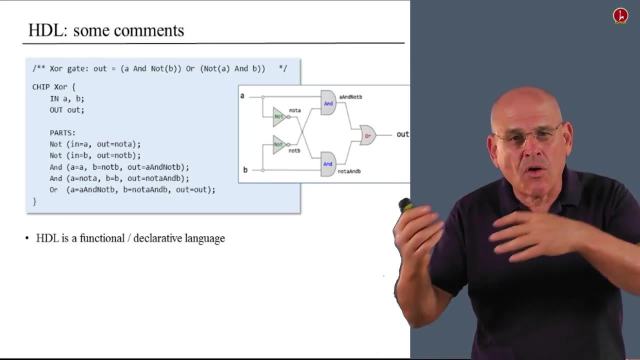 You know it's external To the HDL code. So because HDL is a functional language, we can actually write those HDL statements in any order that we wish. You know, it doesn't matter if you begin to describe the NOT gate or the OR gate. 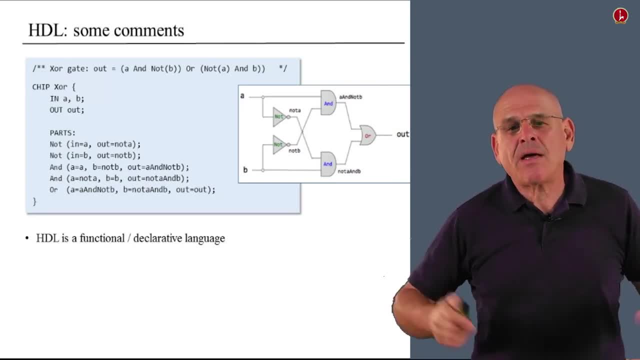 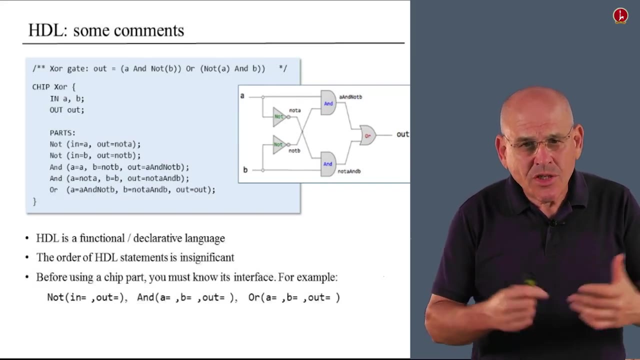 It's completely up to you, But it is typically. it's customary to begin to describe your diagram from left to right, And this also makes the code More readable. Also, note that each time we use an off the shelf gate, we commit ourselves to using the gate interface. 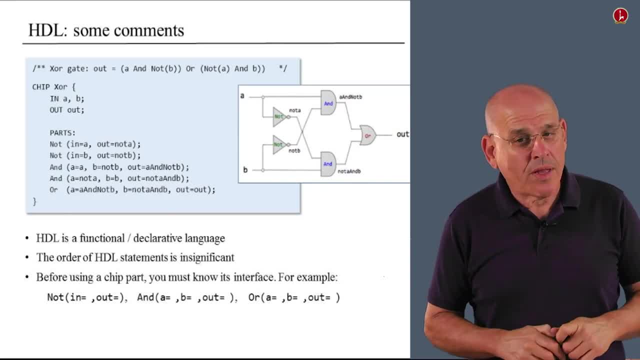 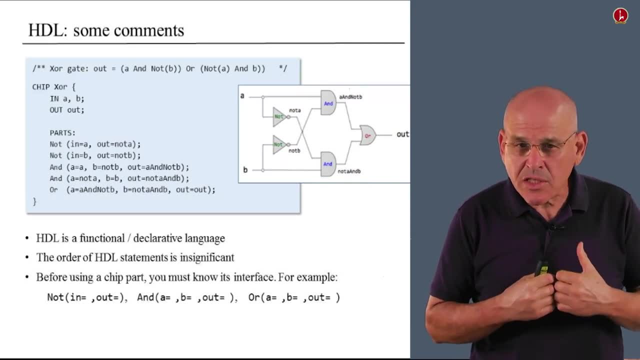 That is the names of the inputs and outputs that come along with the gate documentation. Now, in the hack computer that we're going to build in this course, we decided as a matter of convention to almost always use the letters A and B for a two input chip and out for a single output chip. 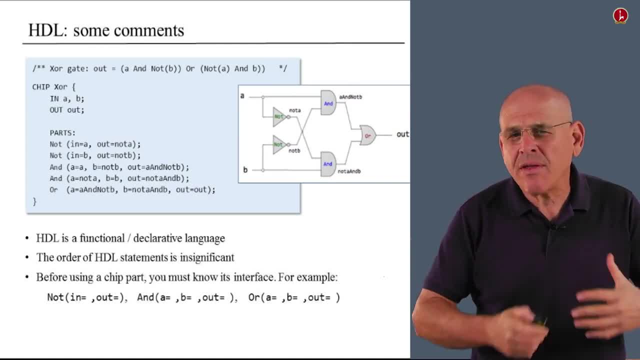 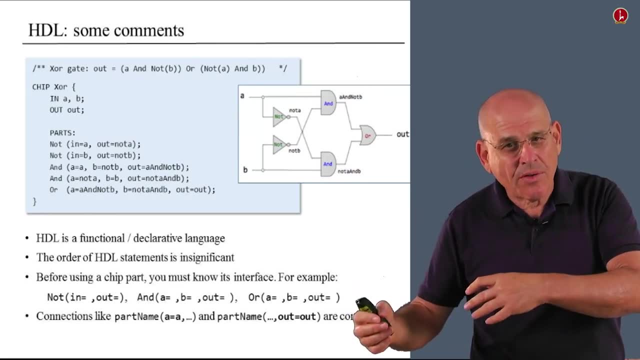 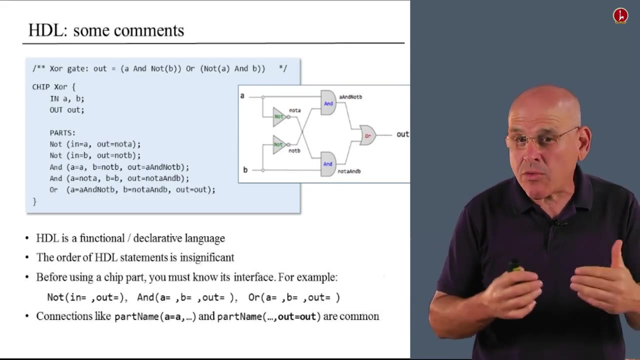 And therefore we are going to have many chip connections that look like A equals A and out equals out. Now, at the beginning, you know this formalism, these conventions will look a little bit strange. You know what does it mean: A equals A, out equals out. 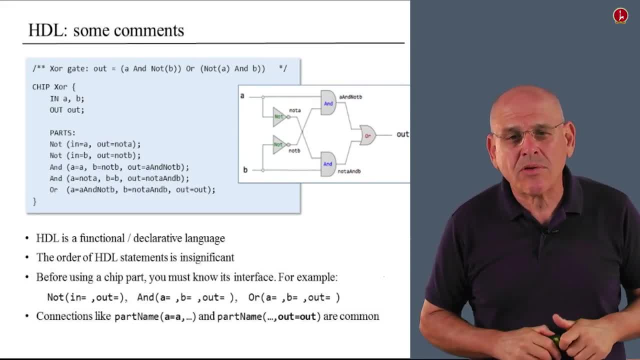 If you think about it a little bit and if you go back to consult these diagrams, you will see that these connections make a lot of sense And actually they are very convenient from a programming perspective. You will realize that once you get your hands dirty and write some HDL code of 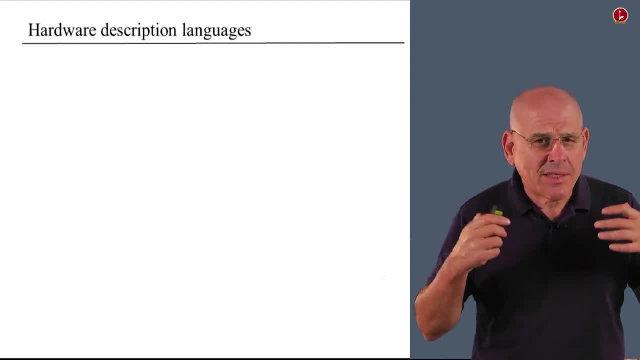 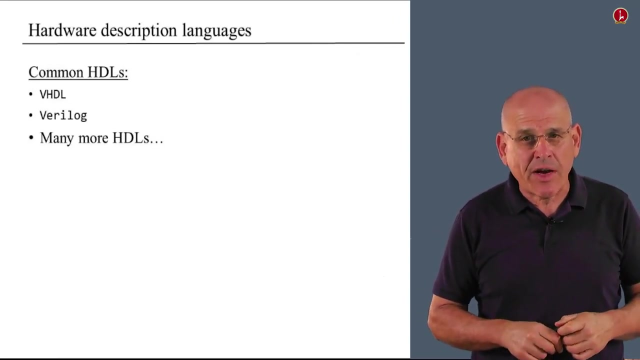 your own. So I'd like to end with some some comments about how the description languages in general. there are many of them out there, and yet the two most popular HDLs that at least I know of are VHDL and Verilog. 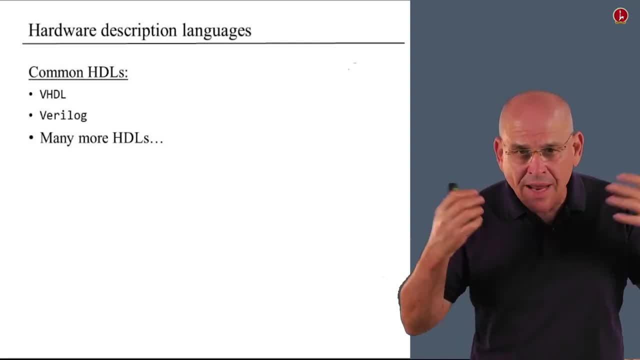 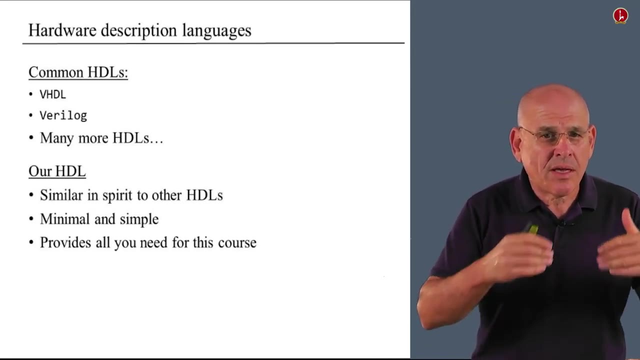 These are the languages which are used, I think, in 90% of hardware design projects, But there are many other HDLs out there that can be used as well. Our own HDL is very similar in its spirit to the industrial strength HDLs that I